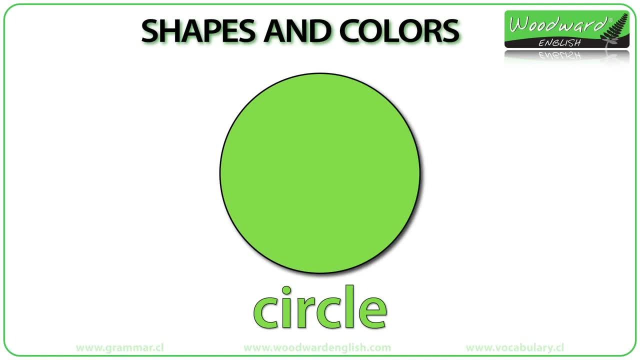 circle, triangle, square, rectangle, oval, diamond, diamond, star, star, heart, heart. What's this? It's a square. What's this? It's an oval. What's this? It's a circle. What's this? It's a diamond. What's this? 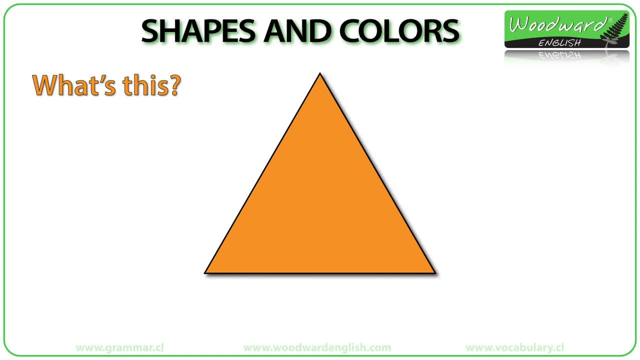 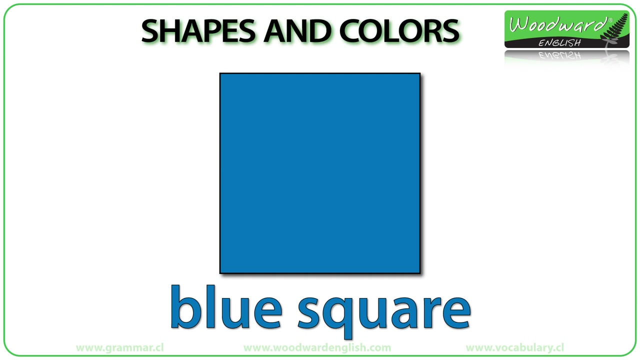 It's a triangle. What's this? It's a heart. What's this? It's a star. What's this? It's a rectangle: A green circle, A yellow circle, A pink triangle, A purple triangle, A blue square. 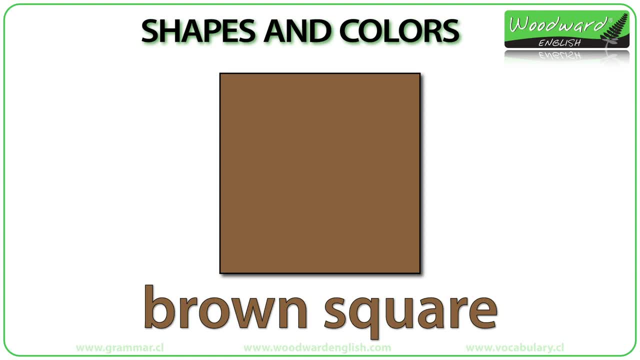 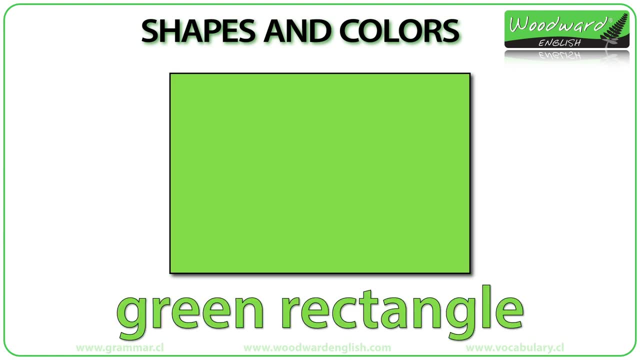 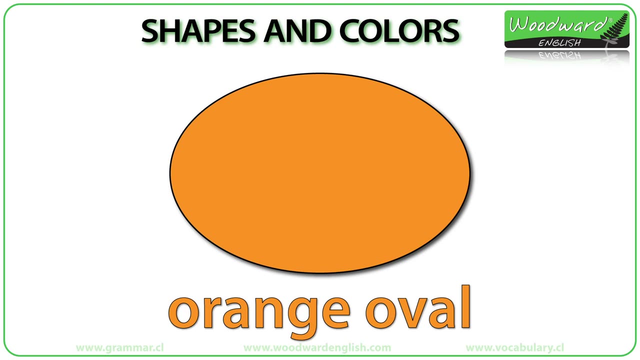 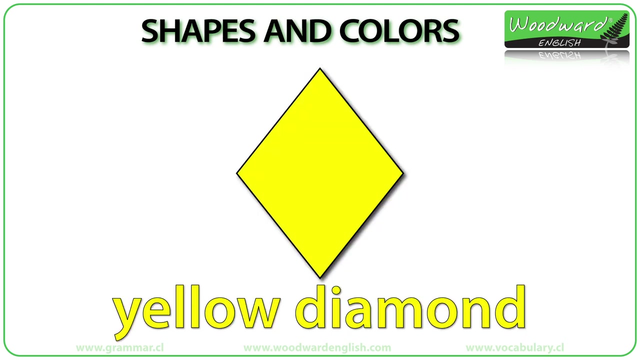 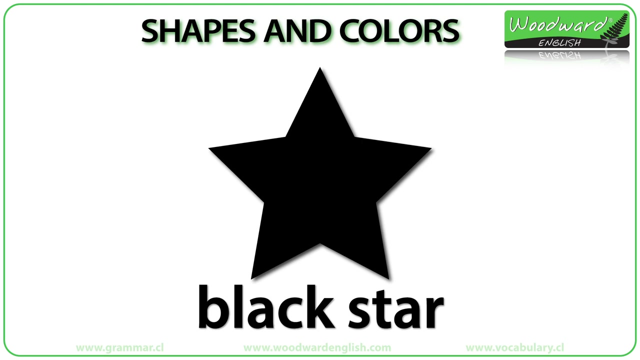 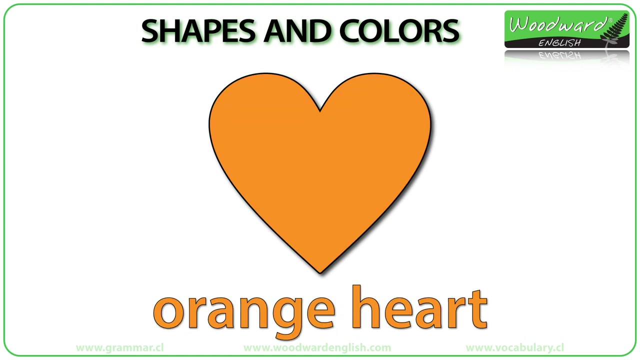 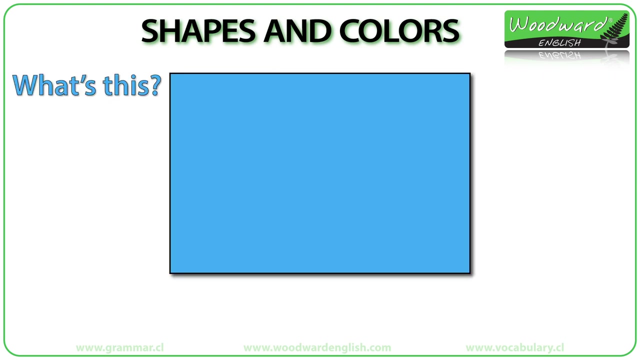 A brown square, A purple rectangle, A green rectangle, An orange oval, A blue oval, A yellow diamond, A red diamond, A white star, A black star, A red heart, An orange heart. What's this? It's a blue rectangle. 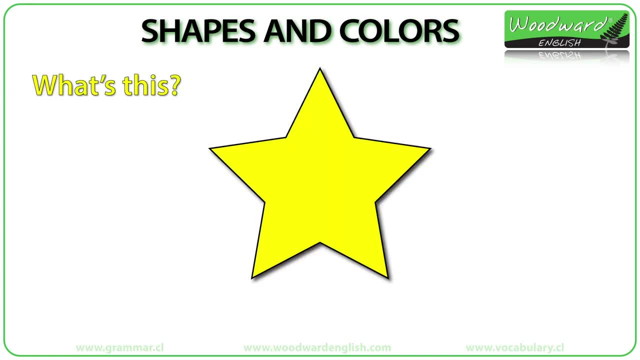 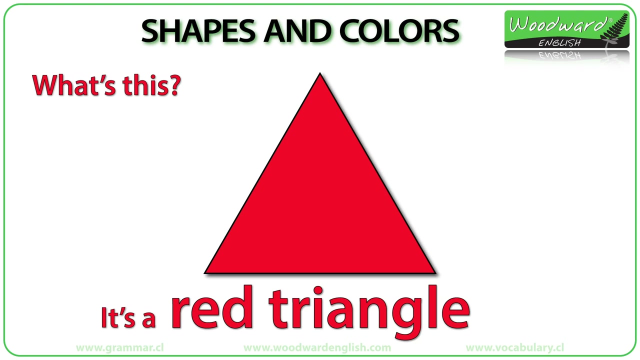 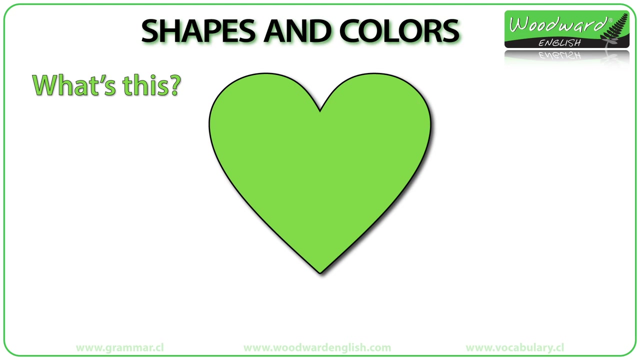 What's this? It's a yellow star. What's this? It's a pink diamond. What's this? It's a red triangle. It's a red triangle. What's this? It's a green heart. What's this? It's a purple circle. 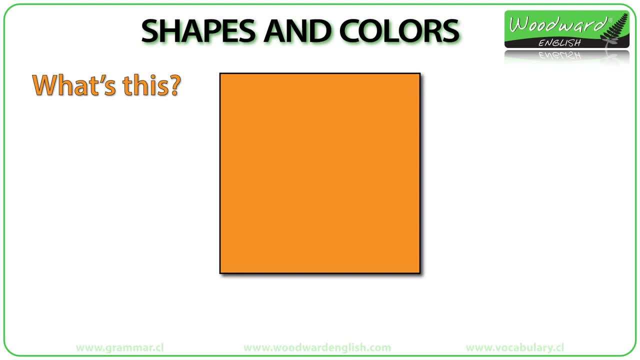 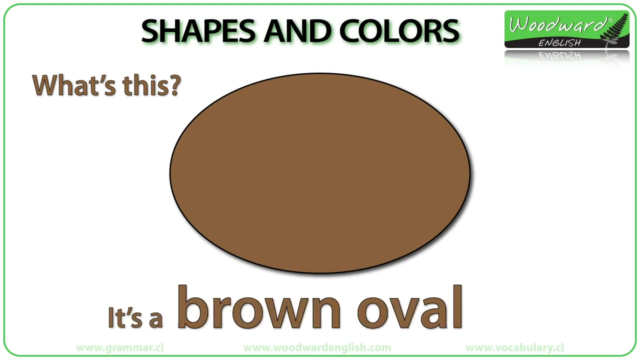 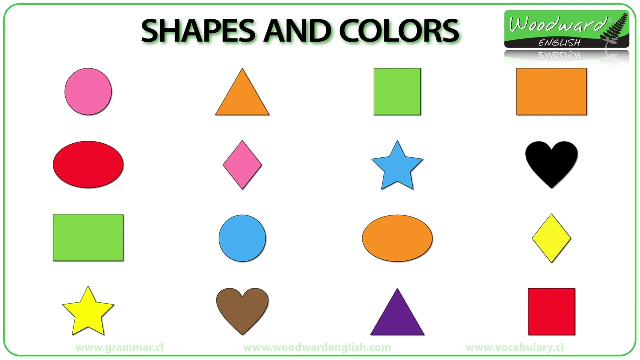 What's this? It's an orange square. What's this? It's a brown oval. Where is the orange rectangle? It's here. Where is the red oval? It's here. Where is the purple triangle? It's here. Where is the yellow star?